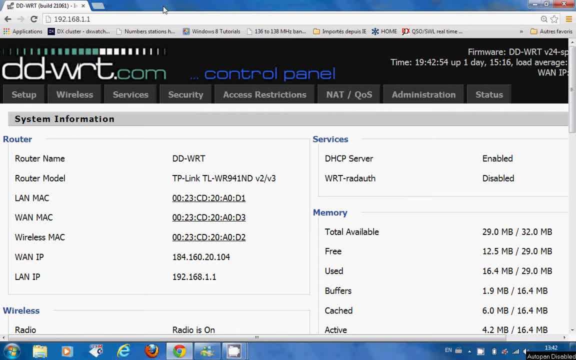 and WPA2.. The WIP standard is an old standard. It's the first security that appeared on routers many years ago and it is to be avoided. WIP is not secure and actually even a neighbor with limited computer knowledge can actually hack into your router and use your internet access using a. 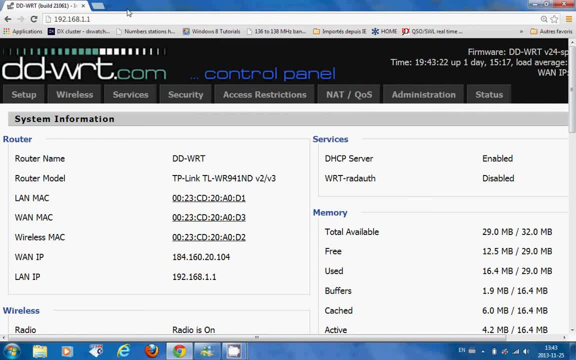 WEP or WEP, So you should avoid this type of protection. The best protection you can use- WPA2, is the latest and, from what we can see, it's pretty strong, as long as you use the maximum encryption and put the longest passwords possible. When you look at your router and you want to see 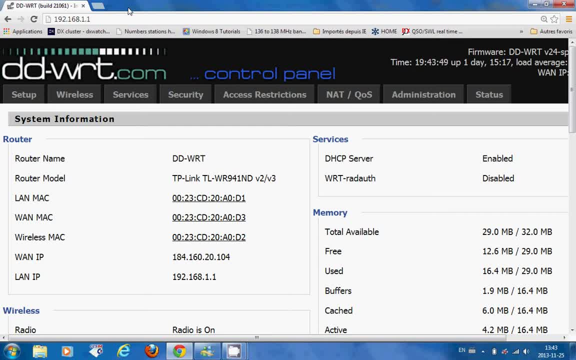 what type of security you're using. you can either use a WIP or a WEP When you use an external device- for example, if you use an iPad, an iPod Touch, an iPhone or even your laptop- will often display the type of security that you have If it says WPA or WPA2,. 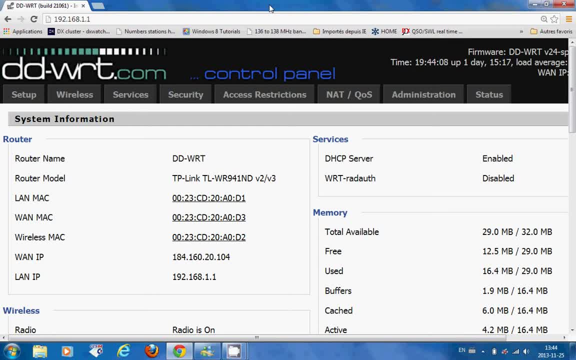 in general, it's safe enough and you should be okay. If you're not sure you can actually login to your router. And how do you do that? Well, first of all you need to know the IP address of your router. In my case, 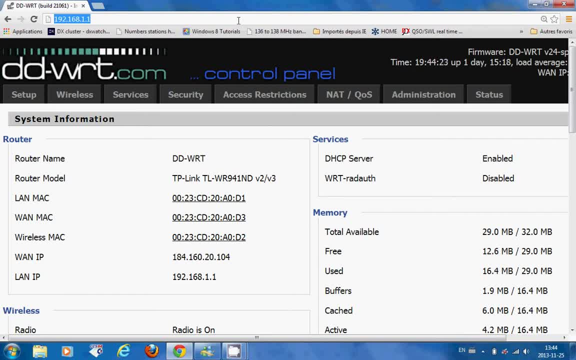 here it's 192.168.1.1. this is pretty standard, so a lot of routers use that IP address. some use a little variant: it's 192.168.0.1. so depending on your model, you can try that in the address. 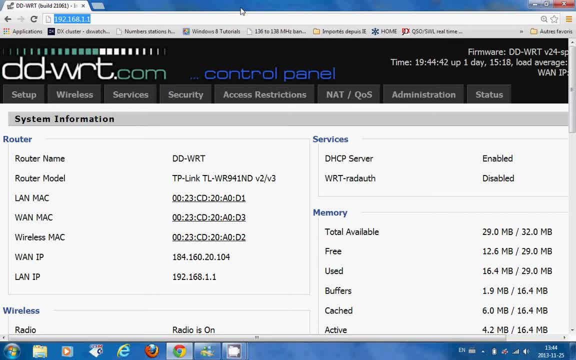 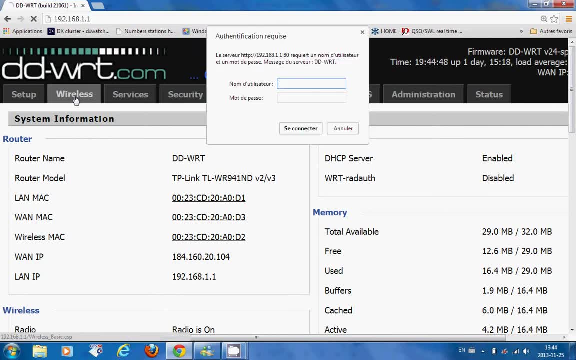 bar of any web browser on your laptop. once you're in your router, you can just go into the wireless section of the router and it might actually prompt you for a username and password. on many devices, admin typed two times, so admin for user, admin for password, preferably you've. 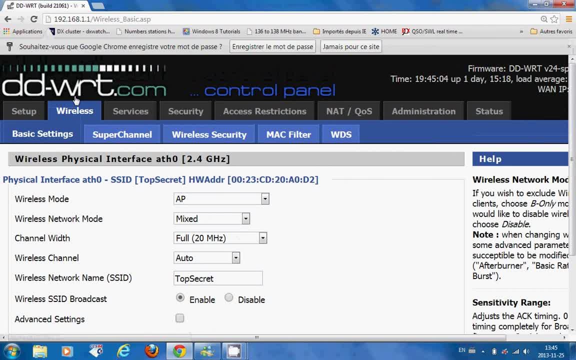 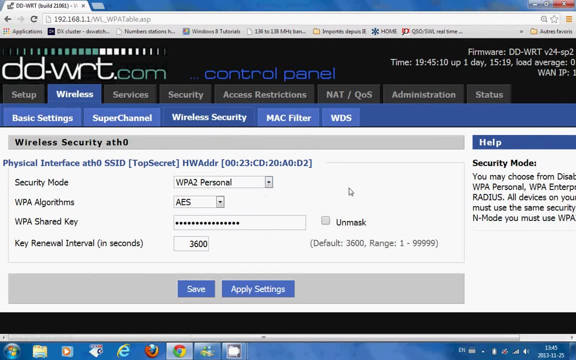 changed this to something better, as I've done. once you're on your wireless, you can go into wireless security and just check the information here. for example, I'm on WPA2 personal and use AES encryption. this is the highest form of encryption available on Wi-Fi routers. usually, if you use 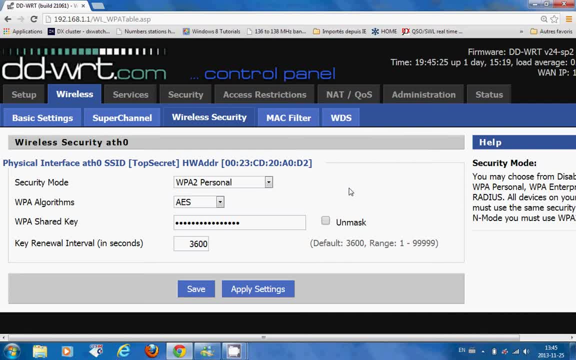 WPA2 and AES. usually if you put a long password- at least 10, 12 characters minimum, and the longer the better- you should be pretty safe and it's going to get pretty difficult to hack into your router. in general, WPA and WPA2 are standards that have evolved and actually have different variations you can. 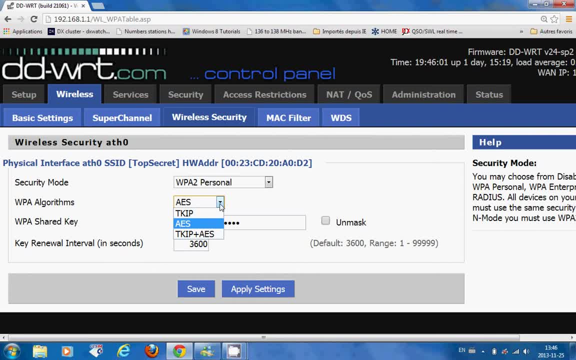 use AES or TKIP, or both can be mixed together. one word of caution: if you use the latest version, that's WPA2, with AES, and you have older devices, there is possibility that you won't be able to connect to your router and you won't be able to connect to your router and you won't be able to. 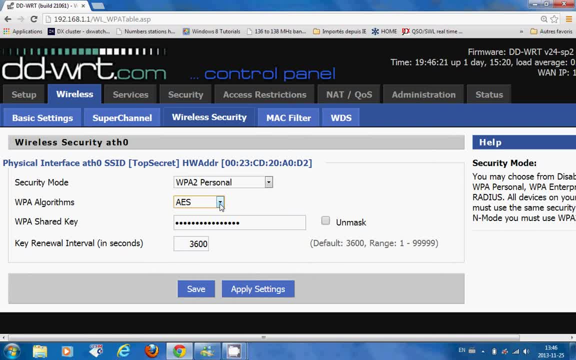 connect to your router because they don't support this type of encryption. my suggestion here is first of all to change AES to TKIP and try if it works. and if it doesn't work then you can actually go back and click and go back to WPA personal so that most devices should connect on WPA personal. 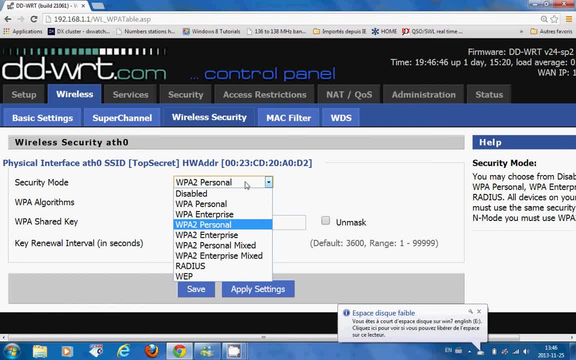 sorry. now, if you have really old devices you can actually connect to your router, and if you have old devices that use WEP, it's kind of complicated. I really, really don't encourage anyone to use WEP keys. I've actually seen a lot of people having the routers act into and their internet connection. 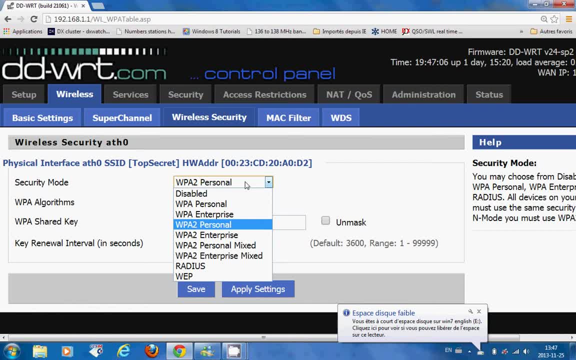 used without their knowledge because they're using the old web standard, so WPA2 should be okay. try to put passwords that are not WPA1 or WPA2 in your router so you can connect to your router, and that are not regular words. you don't want to have any words or names in a.